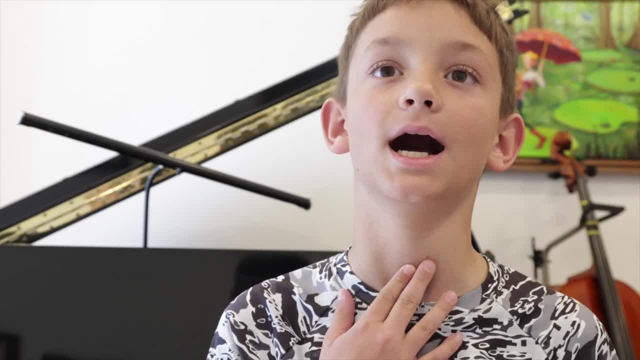 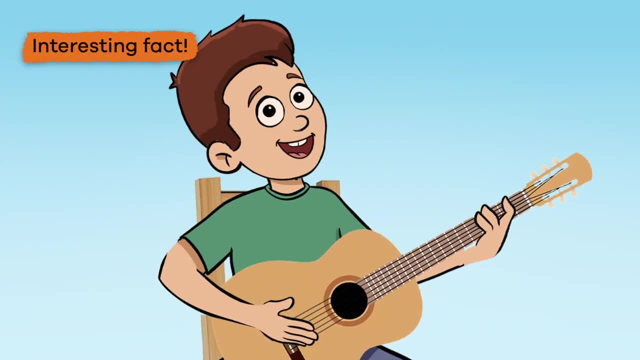 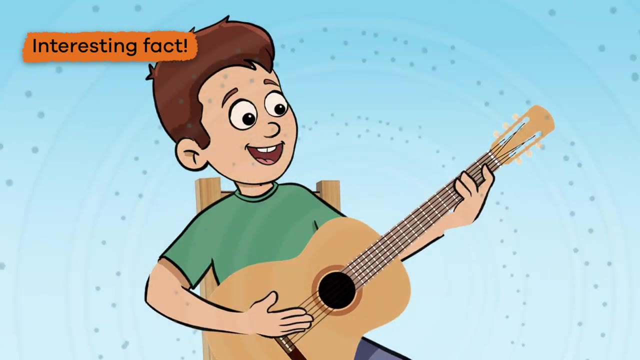 of your throat and hum your favorite song. Do you feel the vibrations of your vocal cords? Pretty cool, huh? Here is an interesting fact: When an object vibrates, it causes movement in surrounding air particles. These particles bump into other particles that are called. 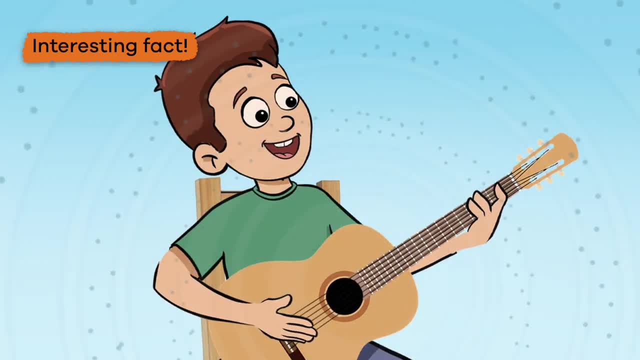 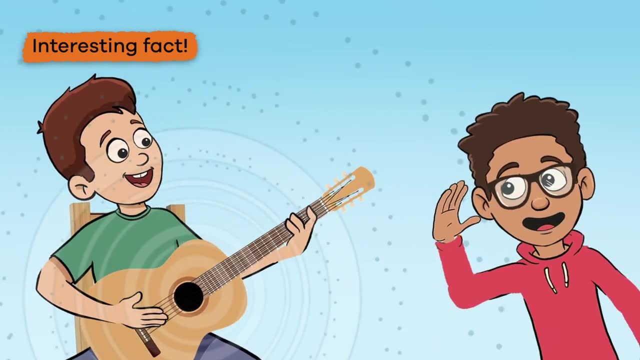 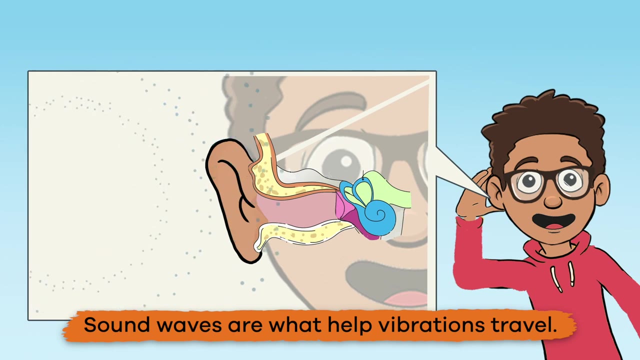 close to them, which makes them vibrate too, And this process continues until the particles run out of energy, kind of like dominoes. This movement is called sound waves. Sound waves are what help vibrations travel, If you are close enough to an object's vibrations. 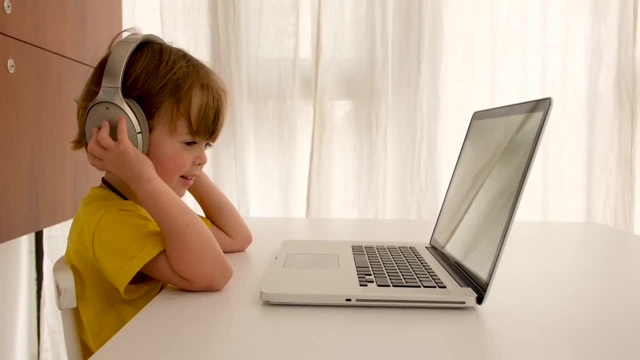 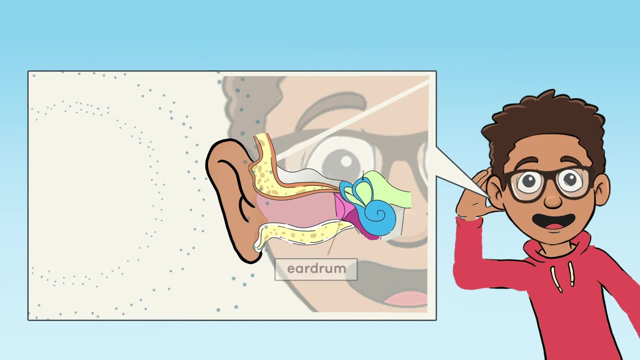 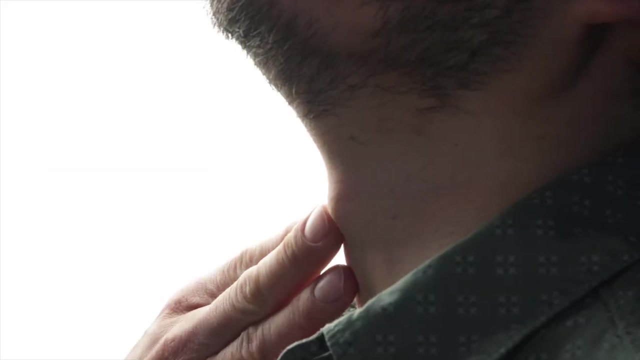 the sound waves that are created will reach your ear. The air particles of the sound waves then vibrate in your ear, which causes your eardrum to also vibrate. This allows you to hear the sound. Now that we know how sound is made and how it travels, let's talk for a minute about pitch and 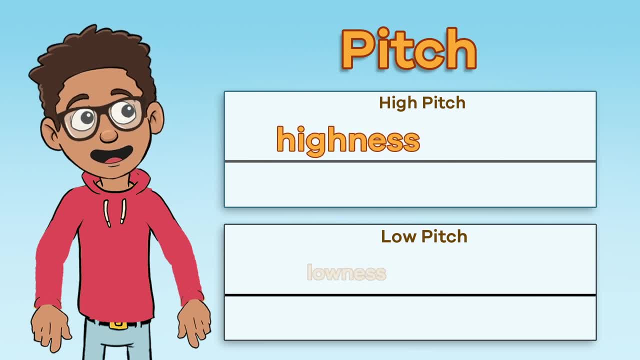 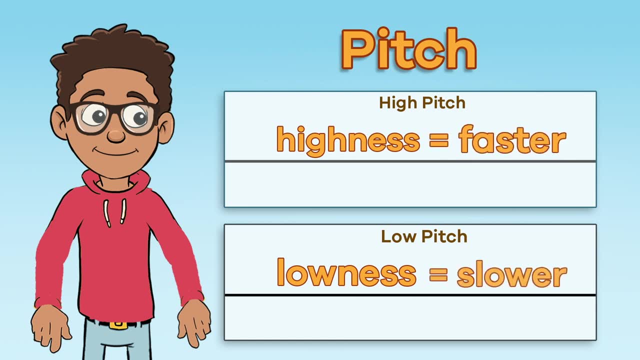 volume. Pitch is the high-ness or low-ness of a sound. Pitch changes when the sound waves go faster or slower. When the vibrations are faster, you hear a higher note. When they are slower, the note is lower. Hey, that rhymes. 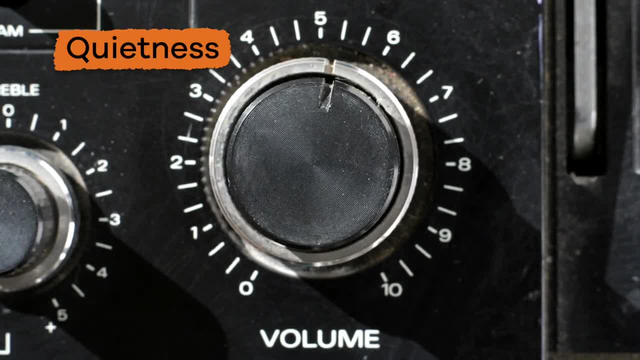 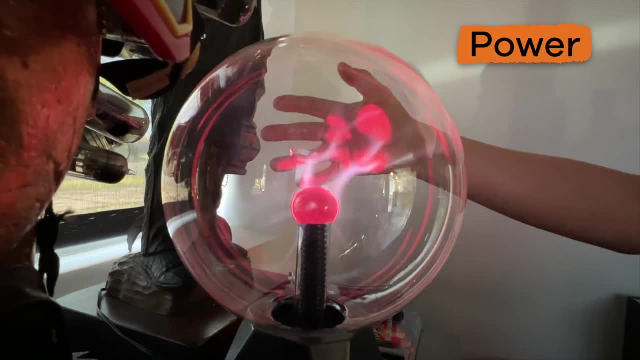 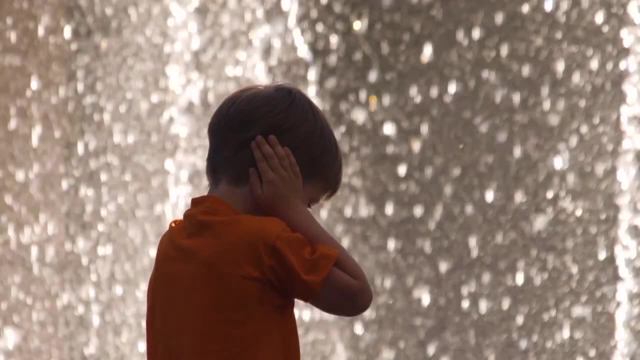 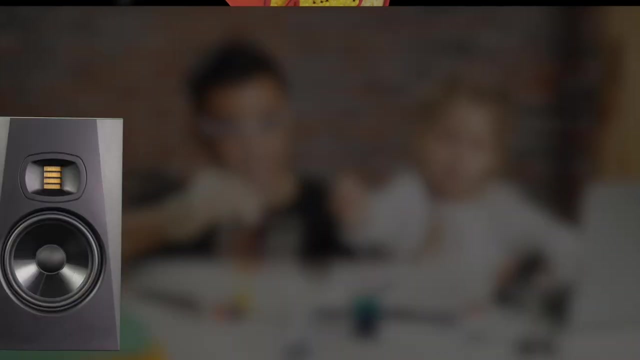 Volume measures the loudness or quietness of a sound. This is called its intensity, which is a fancy way of saying power. The higher the intensity of a sound, the louder our ears hear it and the higher its volume. Volume changes when sound waves are bigger or smaller. 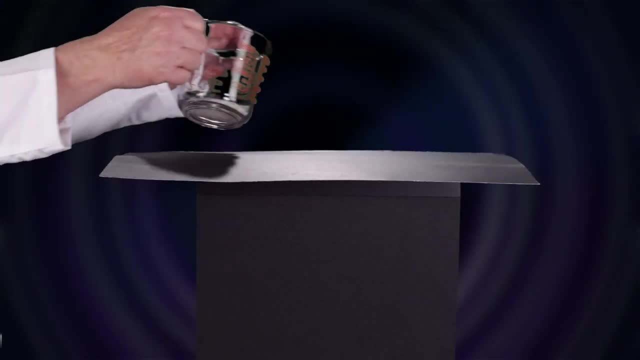 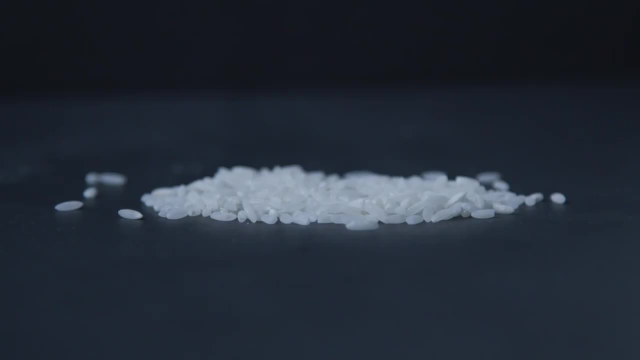 Here is an interesting experiment to try. Place a piece of paper with a handful of uncooked rice on top of a stereo speaker. Turn the speaker on quiet music and watch how the rice jumps Slowly. turn the volume up until the music is really loud. What happens to?